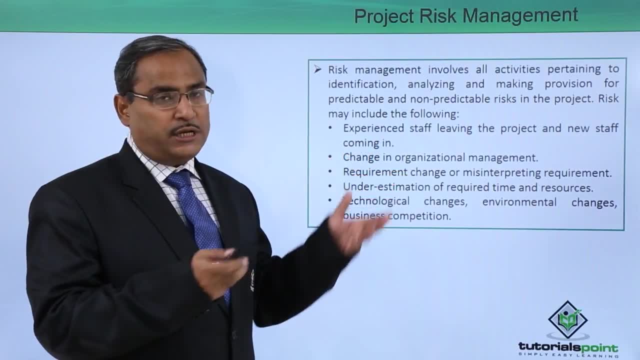 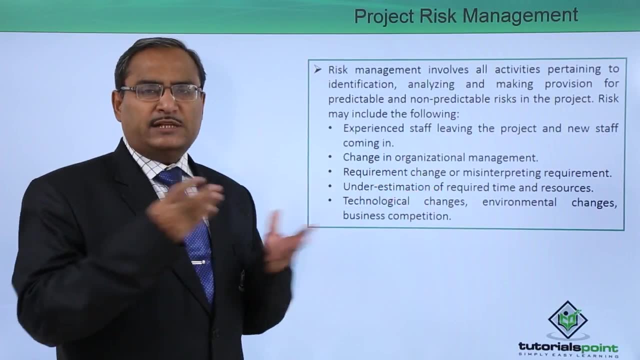 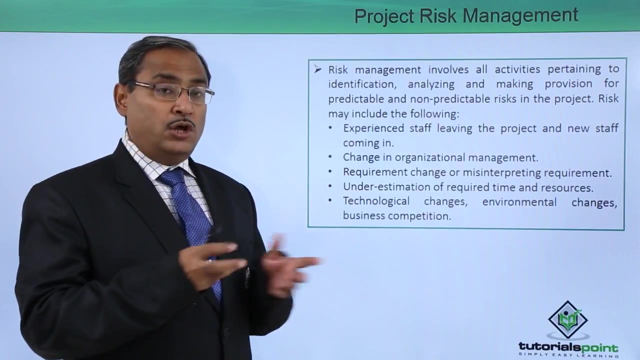 if they leave the respective organization. that will be a very risky affairs. change in organizational management. so top management has got changed. so now they are deploying different rules and regulations. they are changing the rules and regulations so obviously that will cause some risk in the project execution. so requirement change or missed. 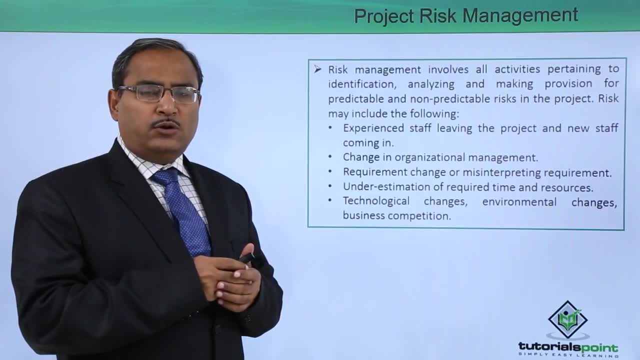 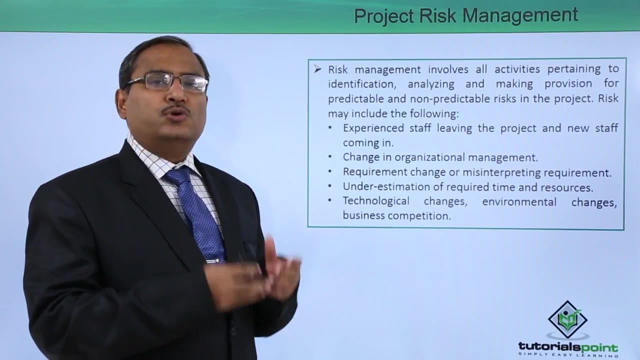 interpreting the requirement. so whatever the requirement that was understood, now it has been found that some misinterpretation is taking place or the requirement is getting changed. so whatever the software we have developed so far, so those new requirements may not get implemented in that very platform. so that is a risky thing. so under estimation of required: 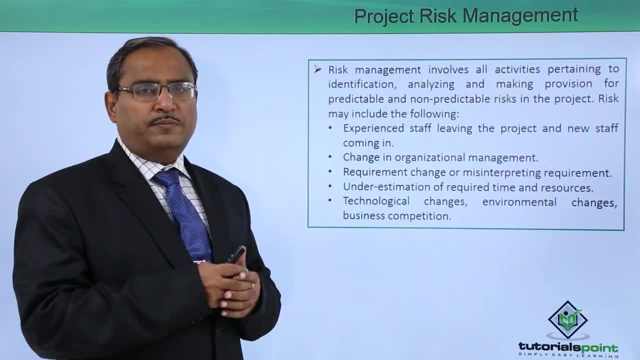 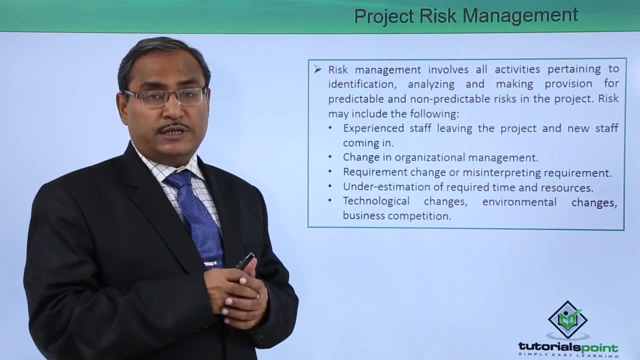 time and resources. so we thought that it will get completed within six months of time, but now we are realizing it cannot get completed less than nine months. i and respective the resources: whatever the resources, whatever the personnel, number of personnel, man hours we calculated earlier, the project execution indicate that we are. 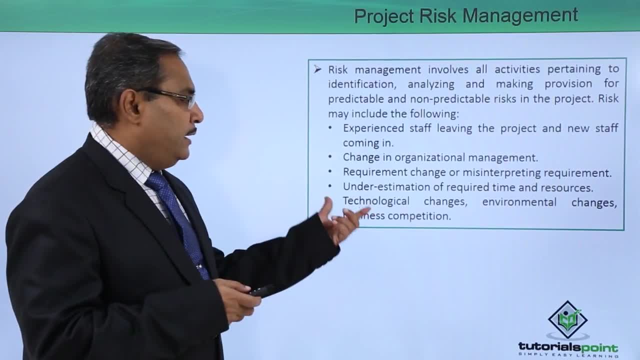 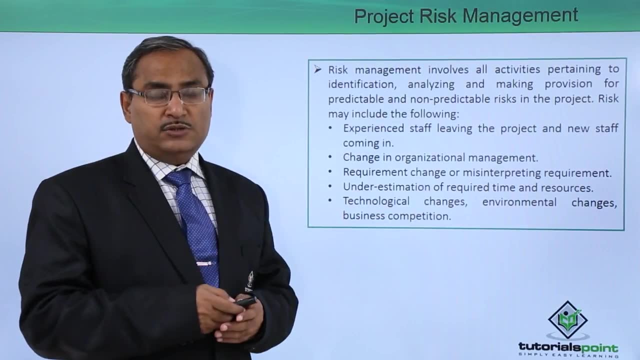 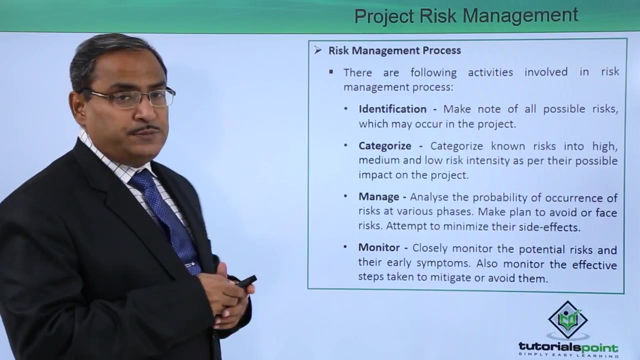 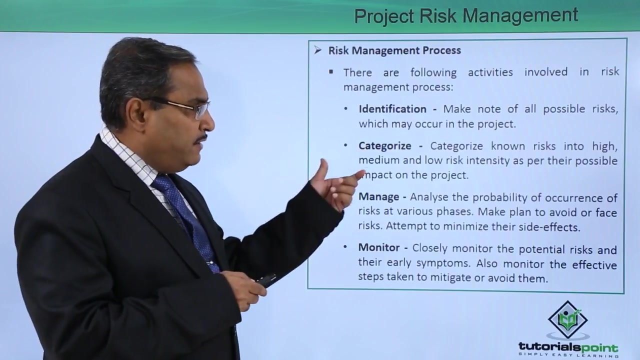 going to miss the deadline, we are going to miss the budget. technological changes, environmental changes and business competition. so these are the different risk factors we usually find in our software project management. so risk management process. so there are following activities involved in risk management process. so what are they? identification, make note of. 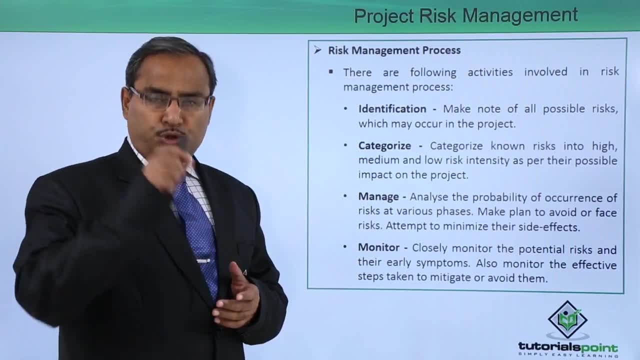 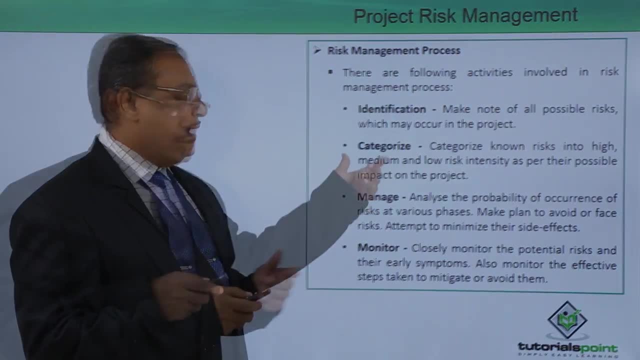 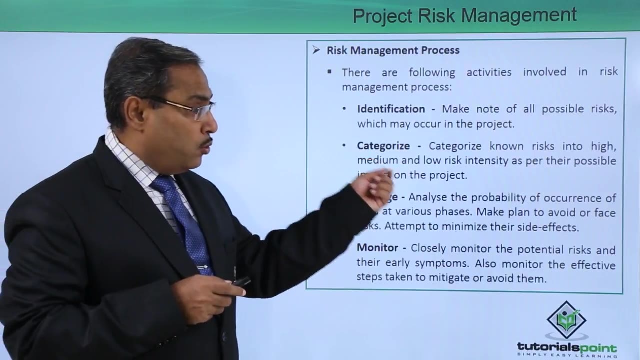 all possible risks which may occur in the project. so we should identify all the risk factors which may come in our project. so you should make a list. next topic is categorized. so categorize known risk to high, medium, low risk intensity as per the possible impact on the project. 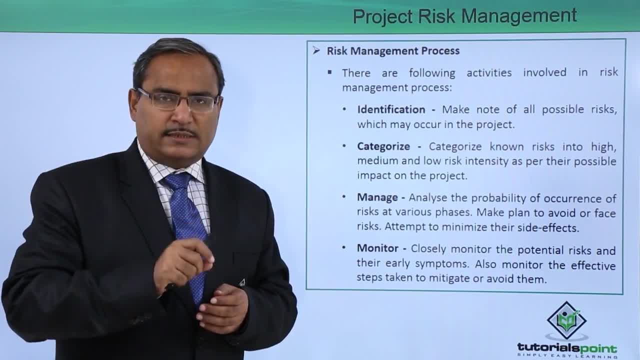 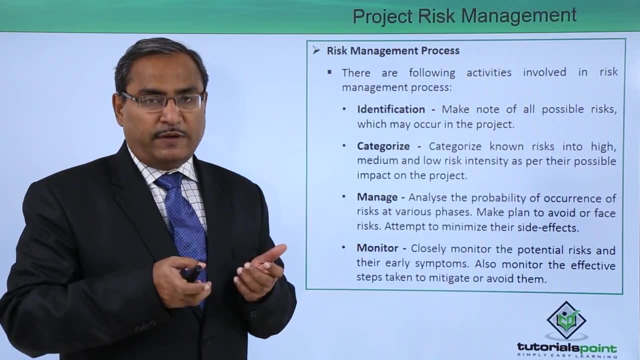 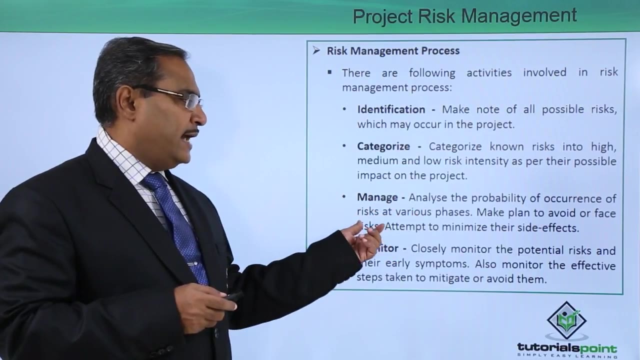 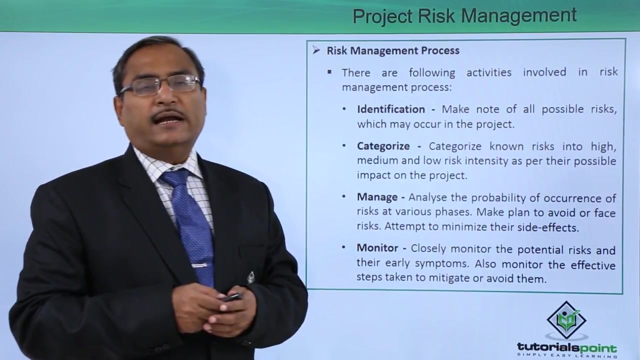 So we are assigning some intensity value on this risks that how much impact this particular risk can have on the project execution, and this intensity values may range from high, medium and low. Manage analyze the probability of occurrence of risk at various phases and make plan to avoid or face risks and attempt to minimize their side effects. So also we. 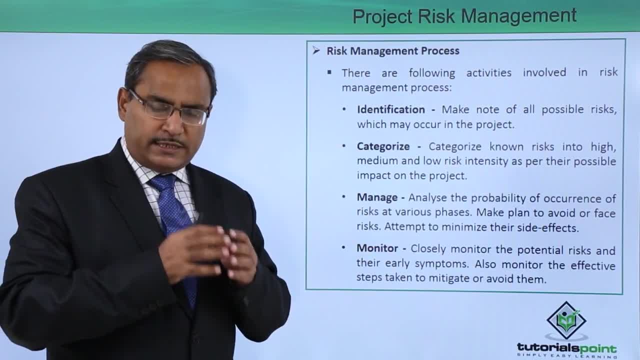 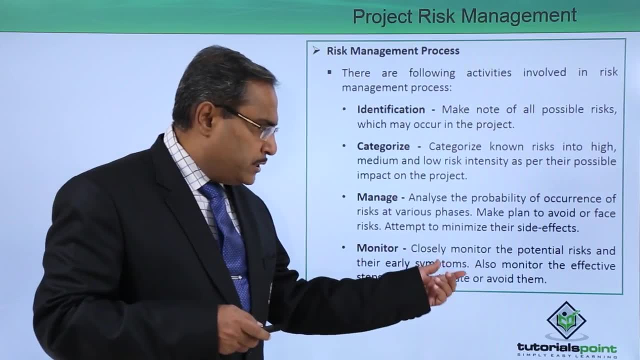 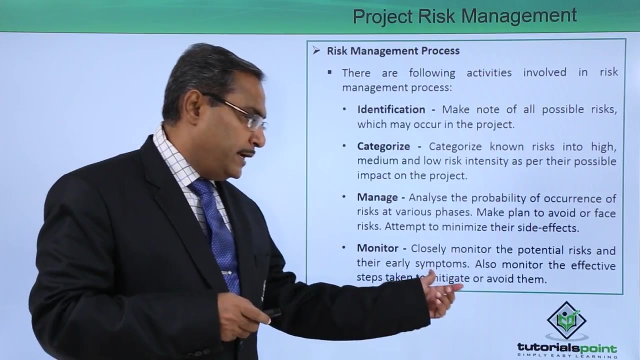 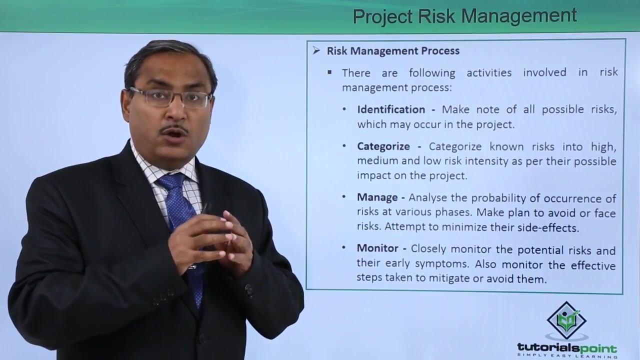 are going to calculate the probability of occurrence of this risks and their side effects. Side effect means unwanted effects. Monitor closely monitor the potential risks and their early symptoms and also monitor the effective steps taken to mitigate or to avoid them. So that means always we should monitor this respective project in such a way that we can. 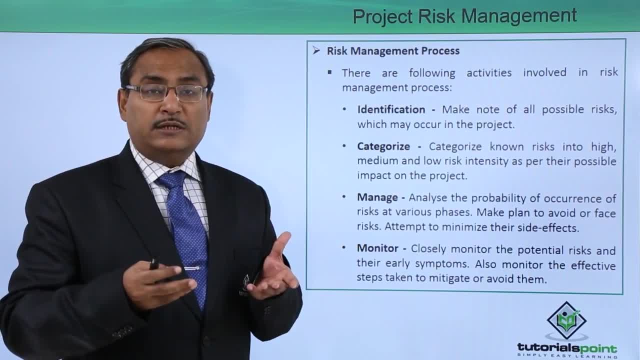 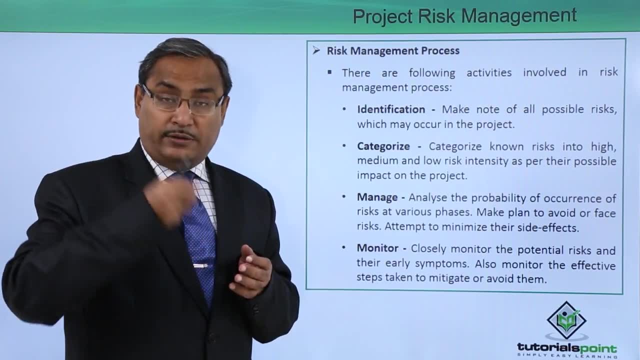 guess that what is going to happen? what are the risk factors? are going to happen, what is going to happen? So we should do the proper monitoring and control so that we can get some symptoms that this particular risk is going to happen. So we should remain proactive. 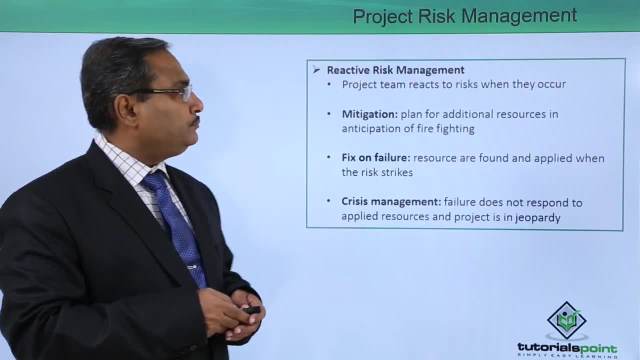 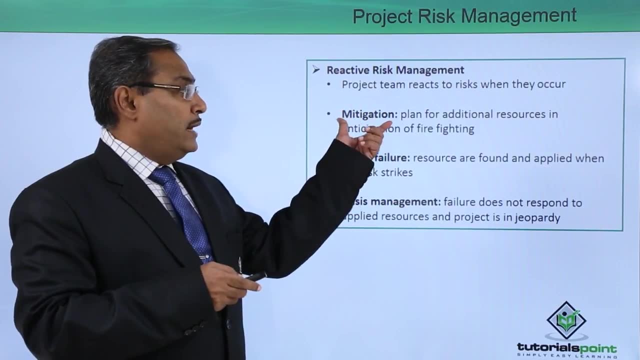 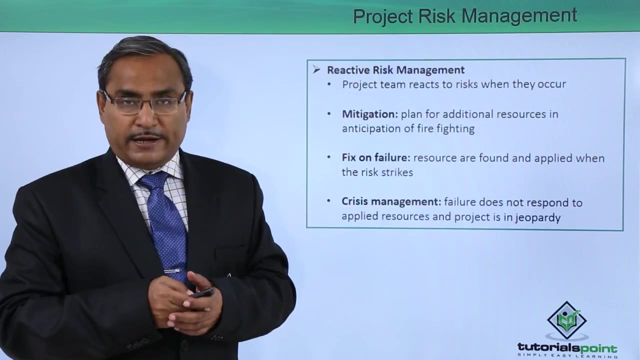 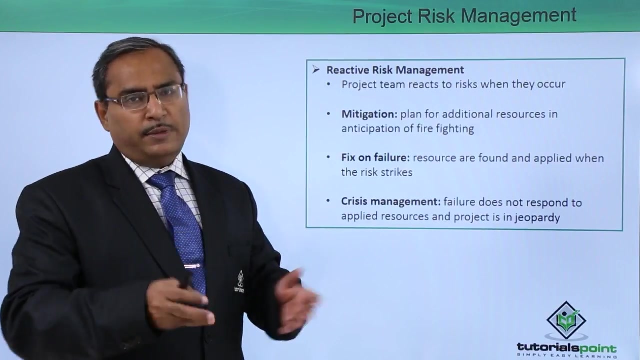 in that case and we should try to resolve that risk. Project team reacts to risk when they occur. Now we are having this mitigation, So plan for additional resources in anticipation of fire fighting. So we should have some reserve resource in our pool So whenever we require them, we can use them in our fire. 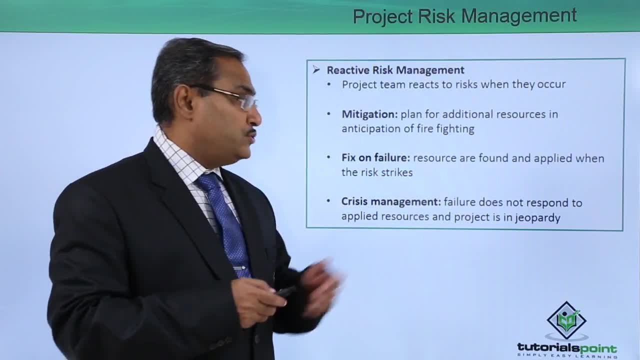 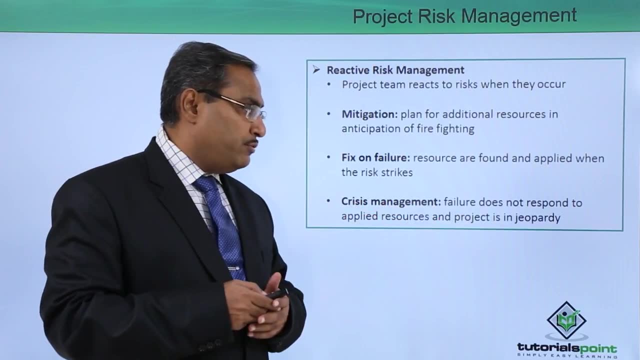 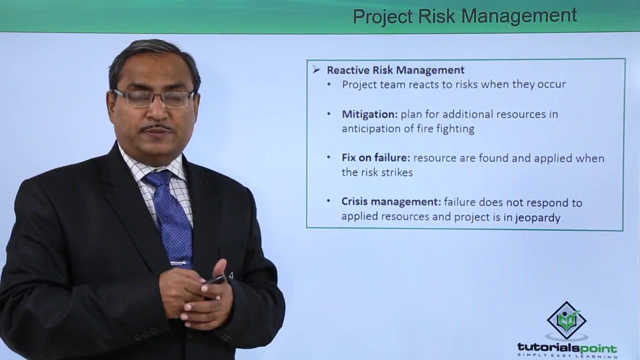 fighting situation. So fix on failure. So resources are found and applied when the risk will strike the system. Crisis management failure does not respond to applied resources and project is in jeopardy. So that means in case of crisis management we have assigned. 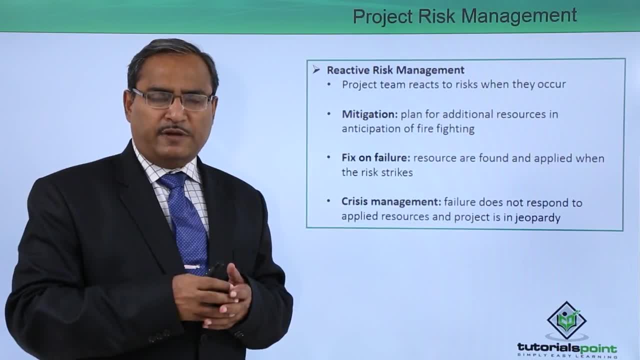 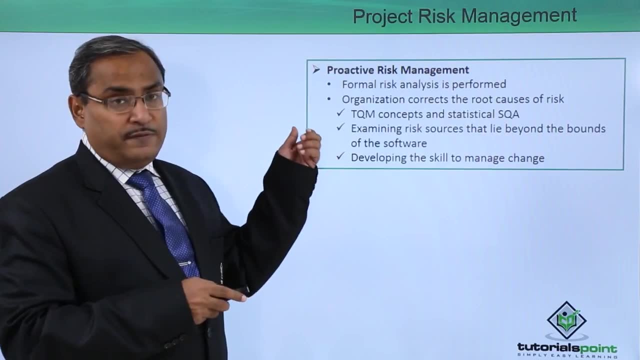 say additional resources, but they are not having any kind of effect in the project, Project progress. So that is known as the crisis management here. So now proactive risk management. So reactive means when the failure has occurred, now what to do, and proactive: 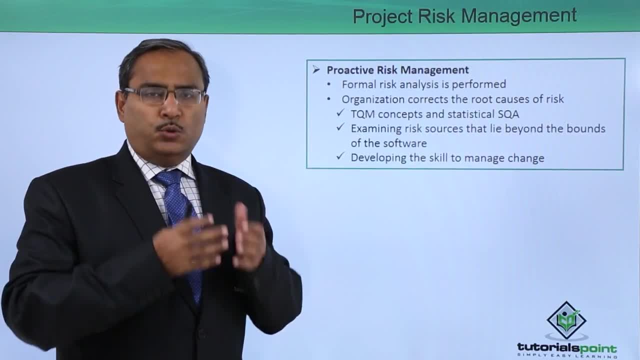 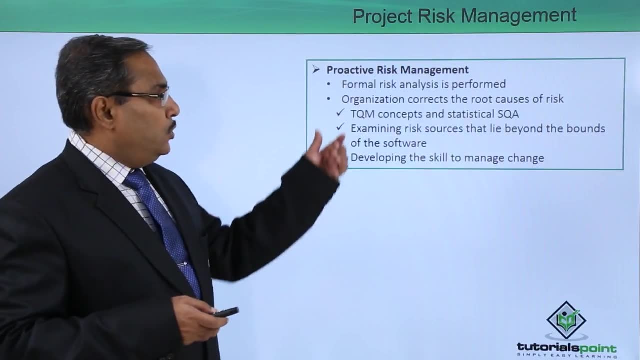 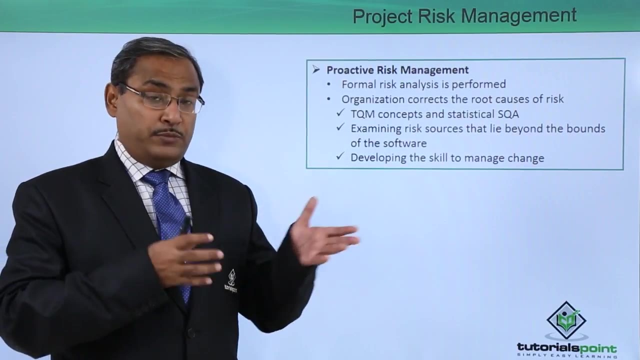 means, after judging the symptoms from our experiences, we should take the preventive measures earlier, prior when the risks are actually occurring in the system. So formal risk analysis is performed. So, whatever the history we are having, so we will be doing the risk analysis and from there we will be having the risk analysis. So we will be 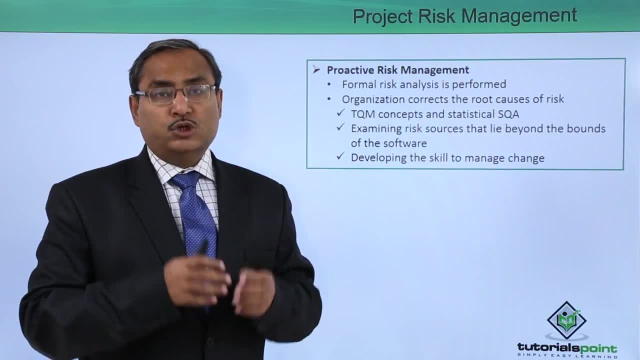 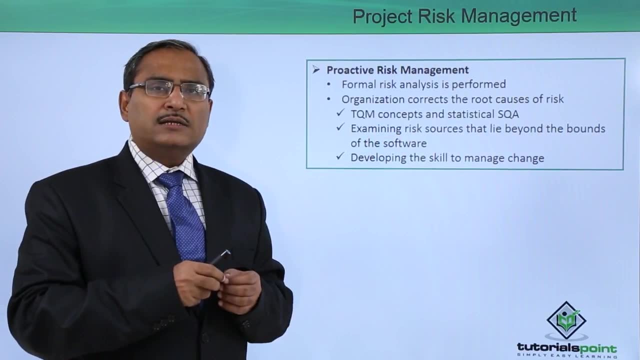 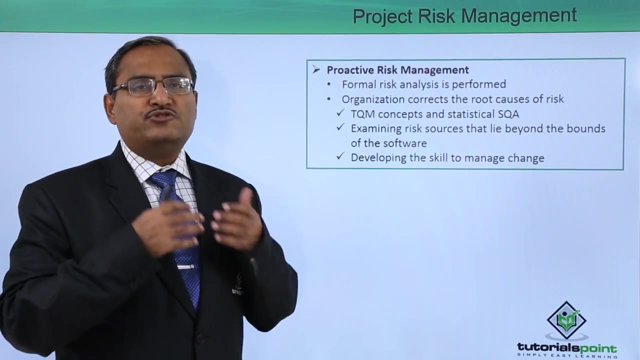 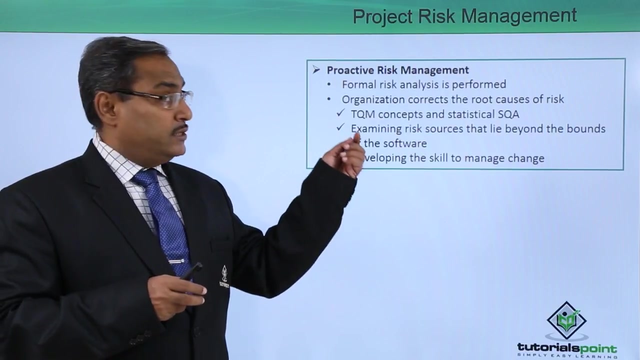 having our prior knowledge and formal risk analysis should be performed and organization corrects the root cause of the risk. That means at first we should go for RCA. What is RCA? Root cause, analysis of different risk factors and organization should do some study on that. and total quality management concepts and statistical. there is a software quality.